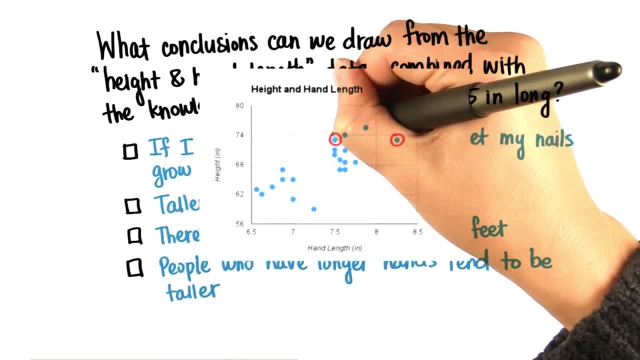 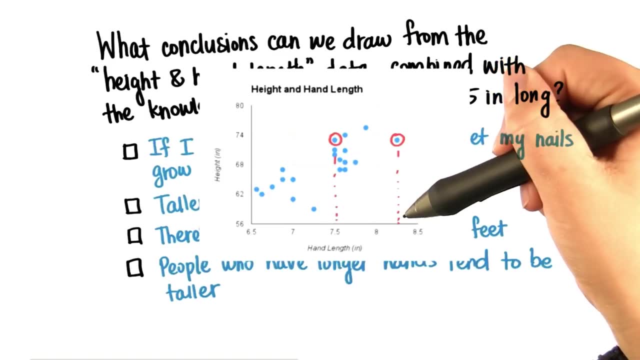 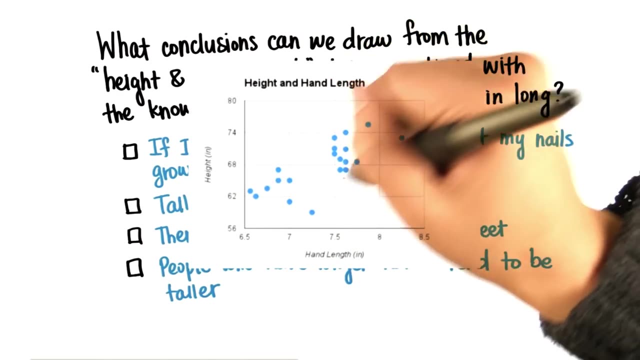 the data, these two people look like they have about the same height, but they have very different hand lengths. Therefore, we can't say with certainty that taller people automatically have longer hands. There's just a trend in that direction. Also, if we look at this trend, we see that people who have about my 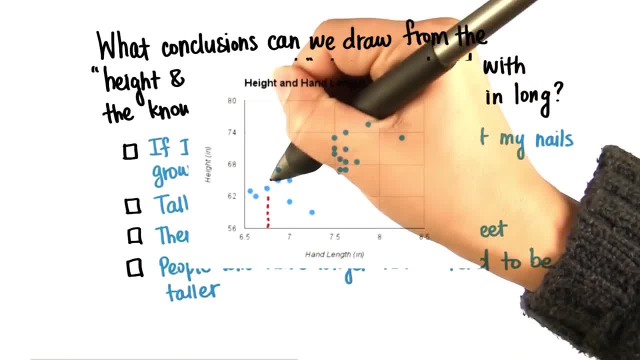 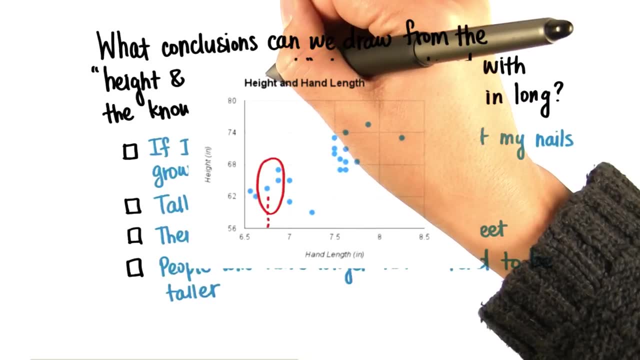 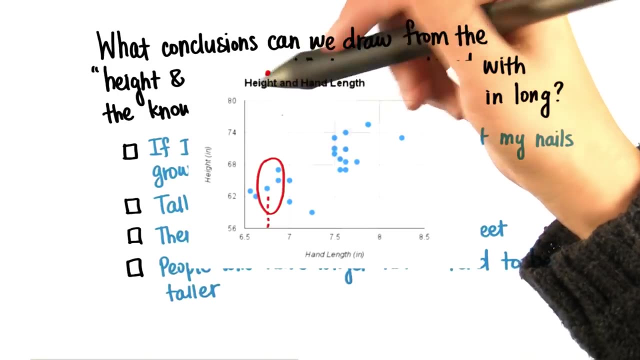 hand length, which is 6.75, tend to have heights around this area. 7 feet is 84 inches, which is way up here. Therefore it's very unlikely that I'm taller than 7 feet, but I could be. Remember. this relationship should be a little bit. 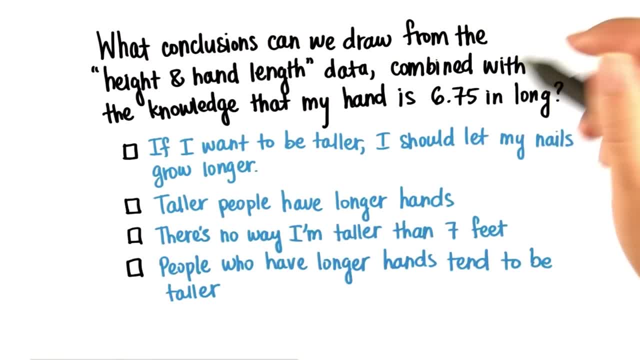 different. This relationship shows a correlation, not a causation. Therefore, we can't draw this conclusion. However, we can say with certainty that people who have longer hands tend to be taller. 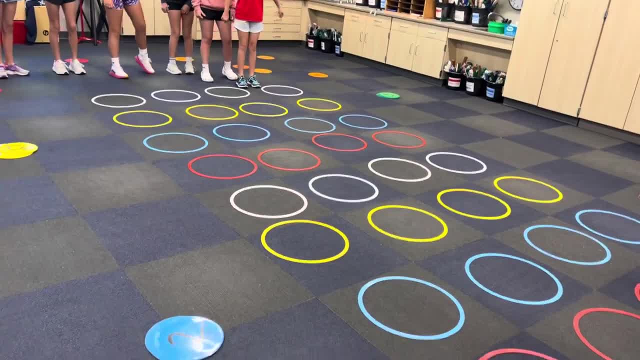 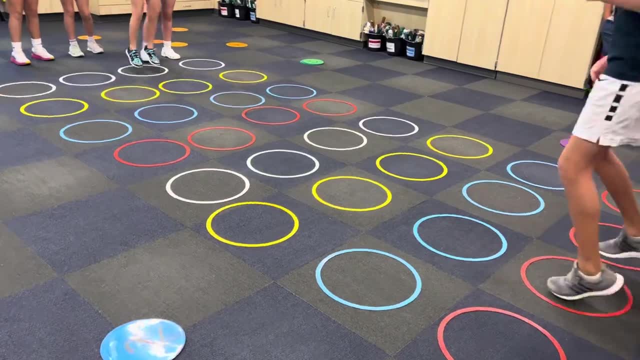 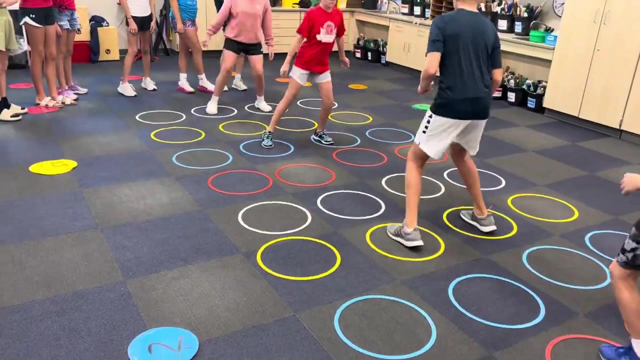 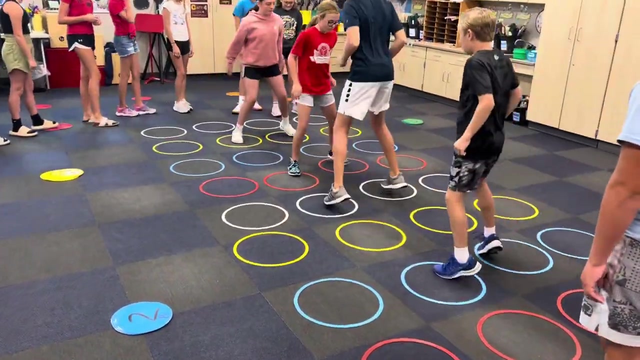 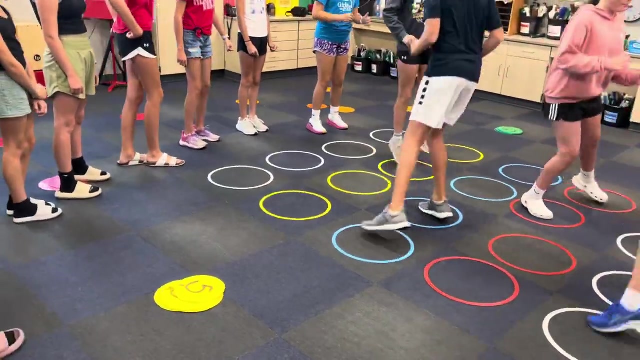 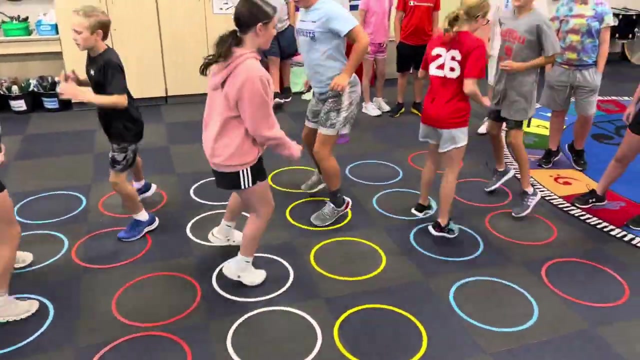 Ready And one, two, three go Front Right, Right, Left, Left Front Right Right, Left, Left Front Right, Right, Left. I love it, It's so good. Left, Left Front Right Right, Left, Left Front Right. 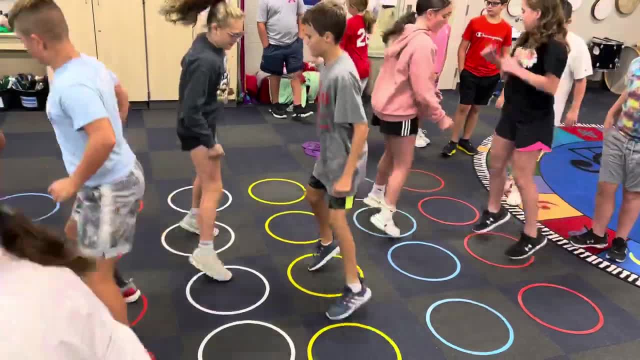 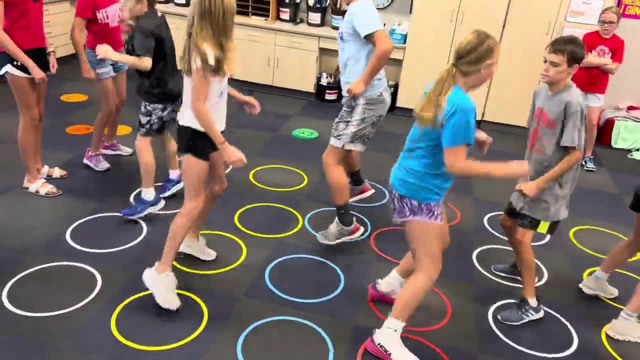 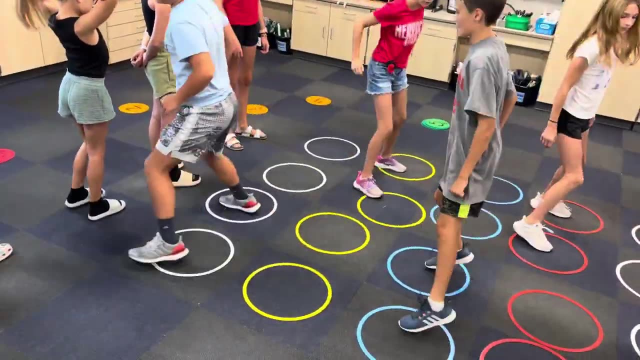 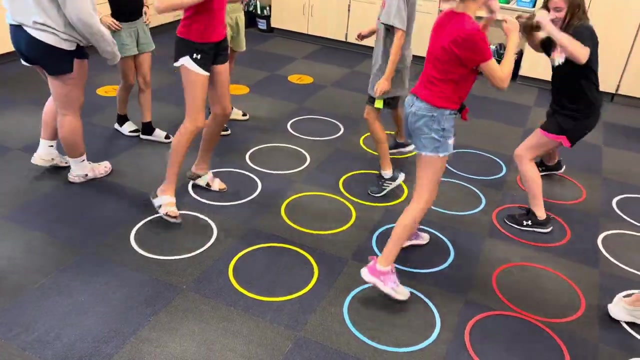